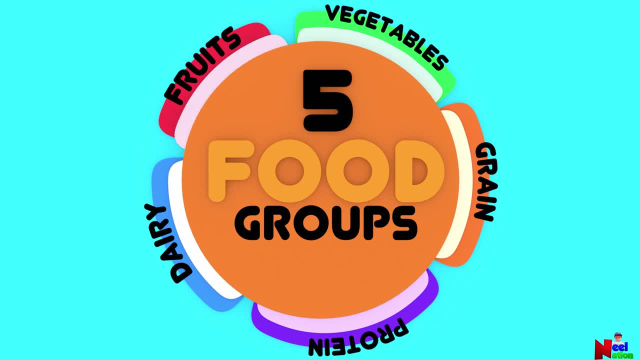 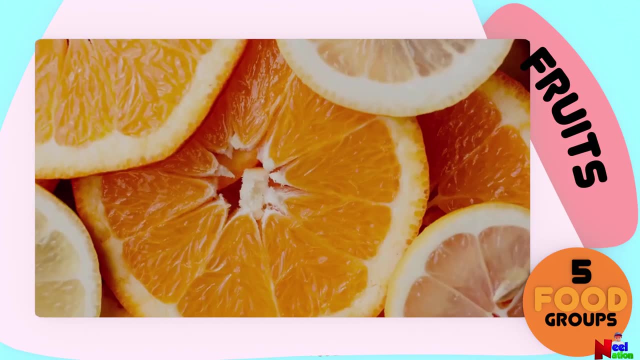 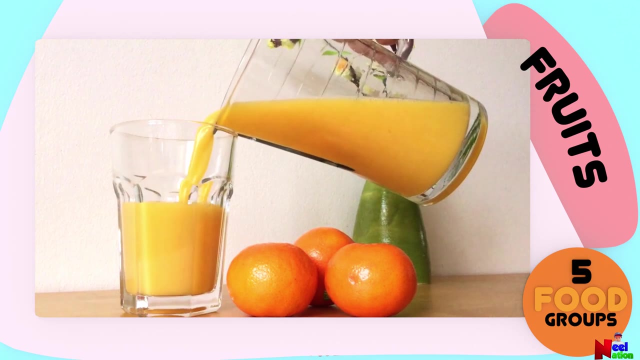 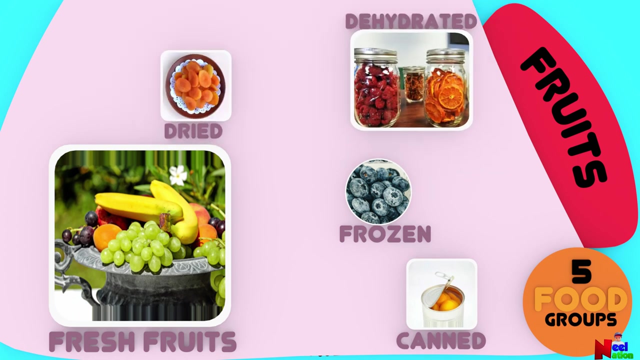 food from these five groups. What foods are in the fruit group? The fruit group includes all fruits and 100% fruit juice. Fruits may be fresh, frozen, canned or dried. Fruits can be eaten whole, cut up, pureed. 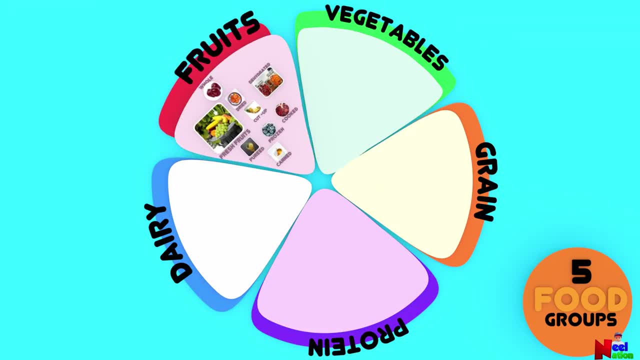 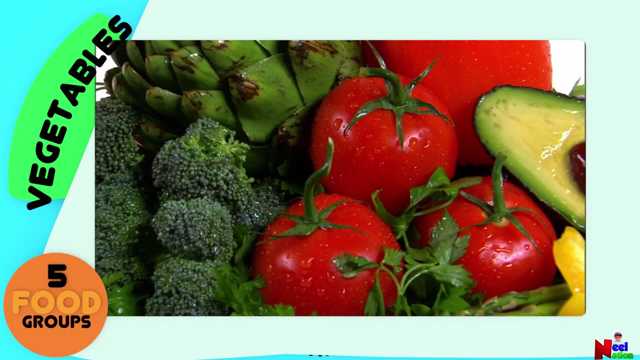 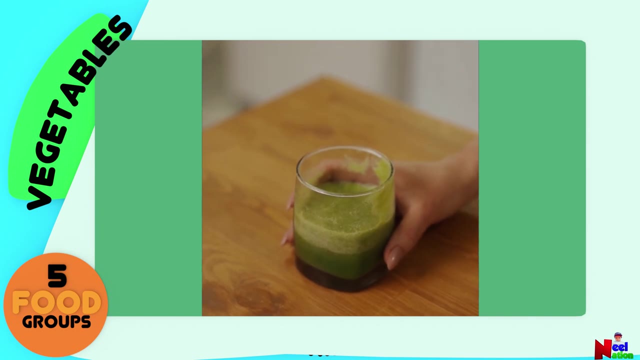 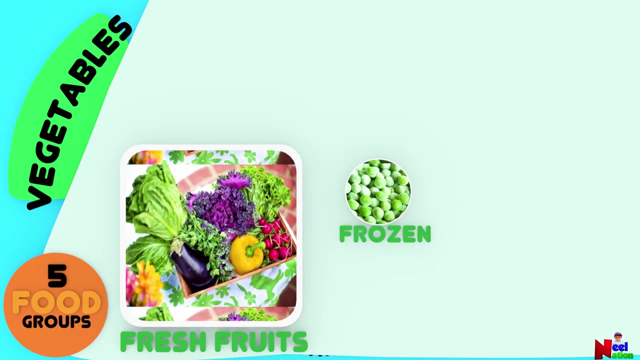 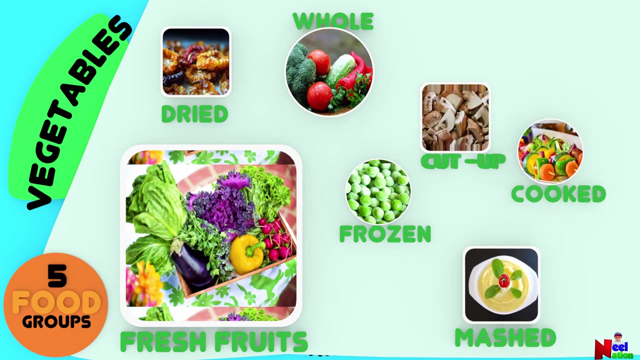 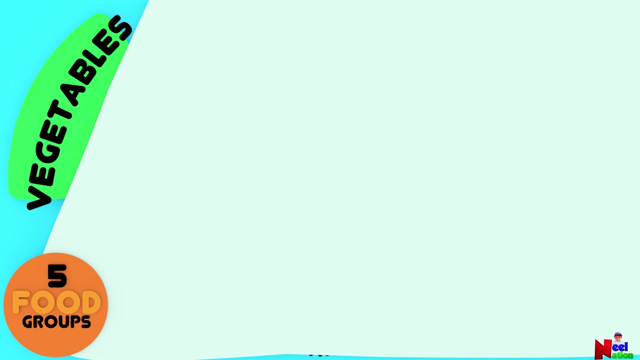 or mashed or cooked. The vegetable group: Any vegetables or 100% vegetable juice counts as part of the vegetable group. Vegetables may be raw or cooked and can be fresh, frozen, canned or dried. They can be whole, cut up or mashed. Vegetables are organized into 5 subgroups based on their nutrients. 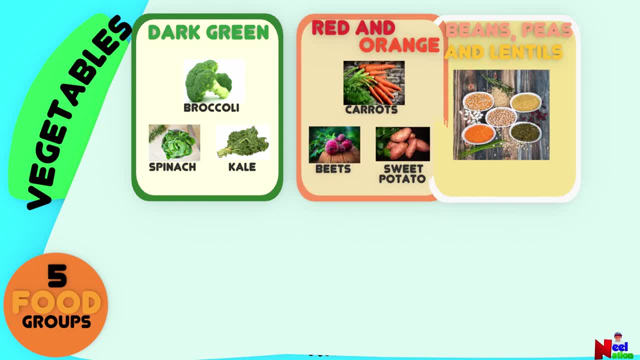 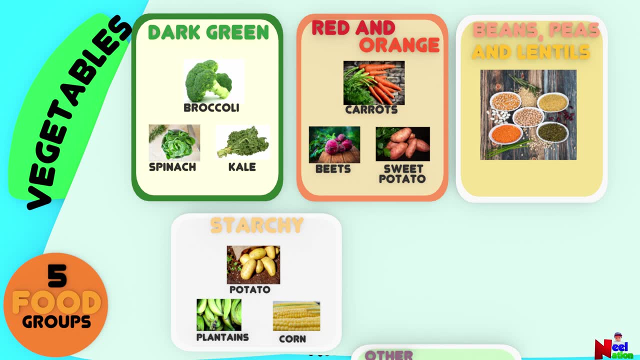 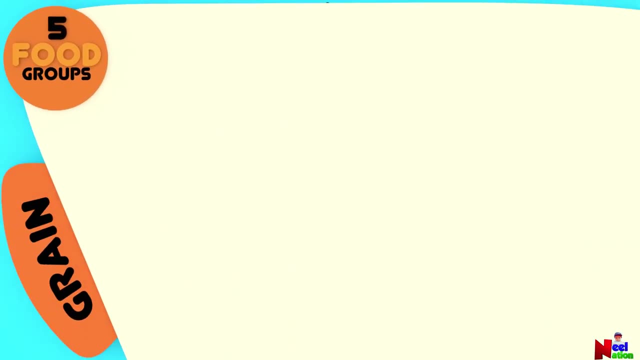 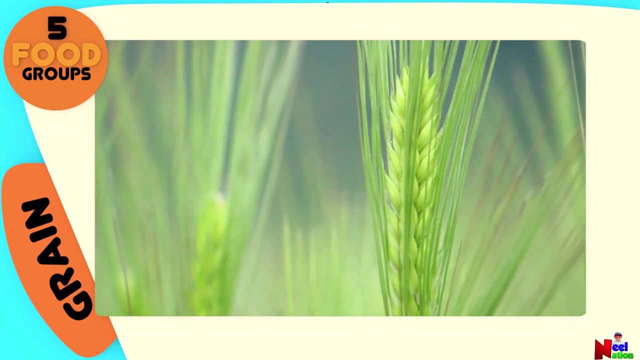 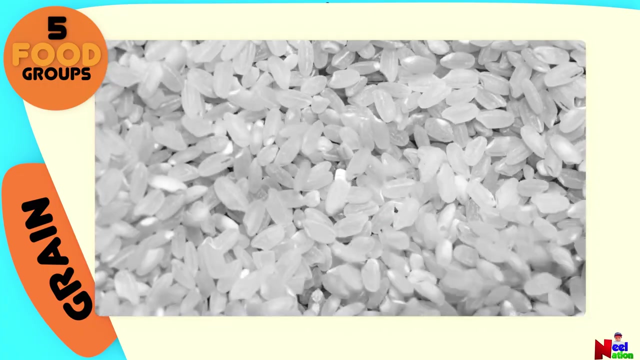 Dark, green, red and orange beans, peas and lentils, vegetables, starchy and other vegetables. The grains group Grains are small, hard and edible dry seeds that grow on grass-like plants called cereals. Grain products made from wheat, rice, oats, cornmeal, barley or another cereal grain. 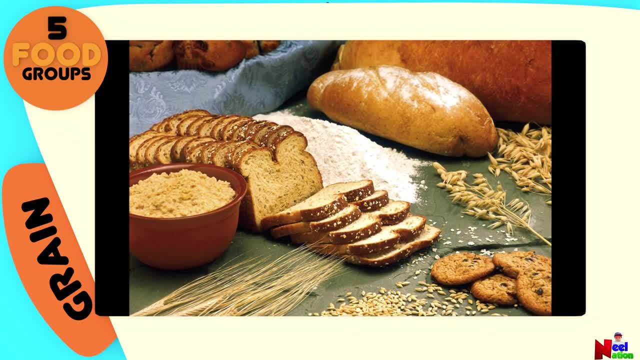 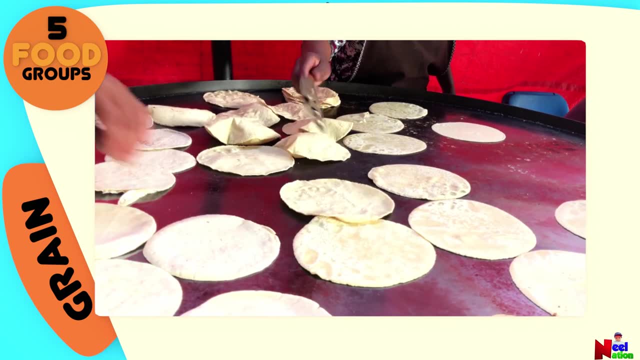 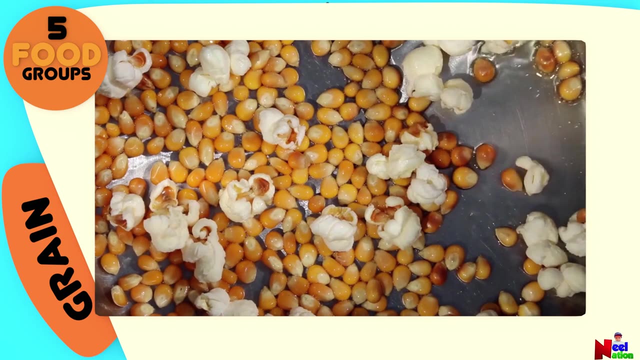 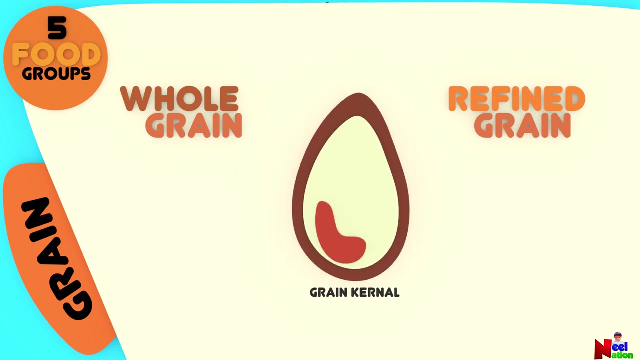 is a grain product. Bread, pasta, breakfast cereals, grits and tortillas are examples of grain products. Did you know that popcorn is also included in the grains group? Grains can be classified as either whole or refined. A whole grain consists of three main parts. 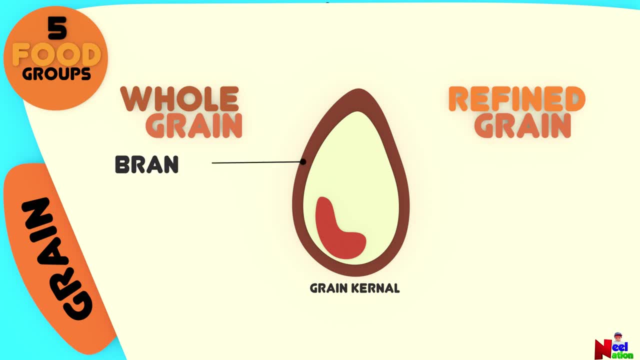 Bran, the hard outer layer of the grain. It contains fiber, minerals and antioxidants. Germ, the nutrient-rich core, is the embryo of the plant Endosperm, the biggest part of the grain. It contains mostly carbs in the form of starch and protein. 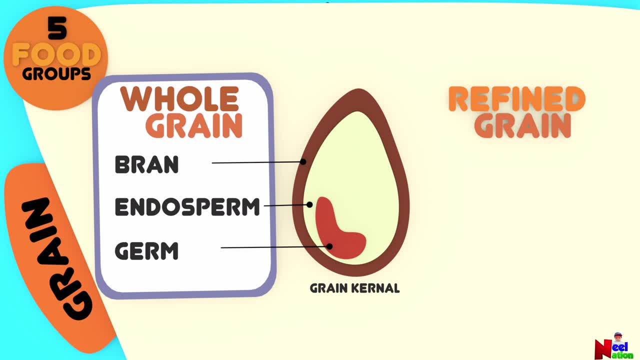 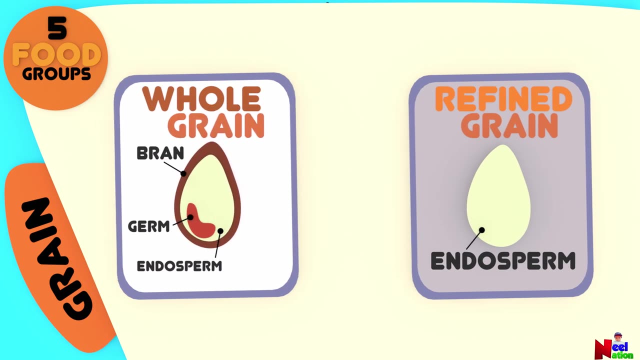 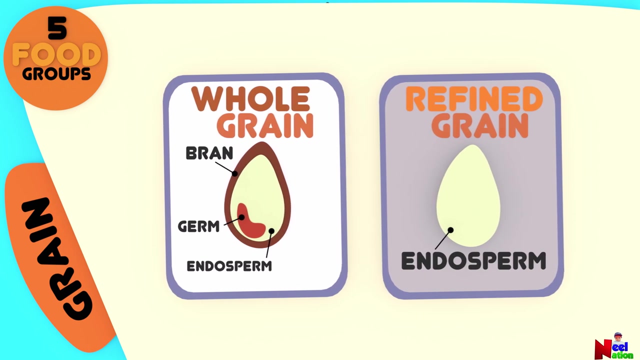 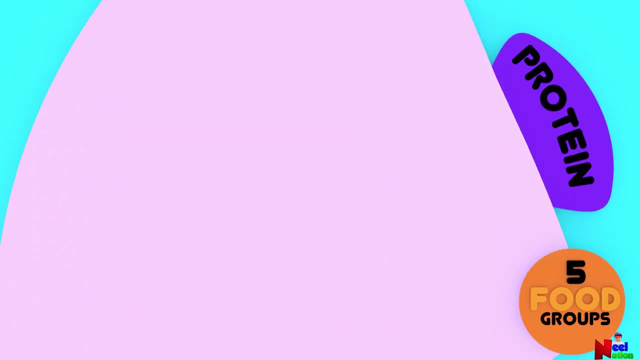 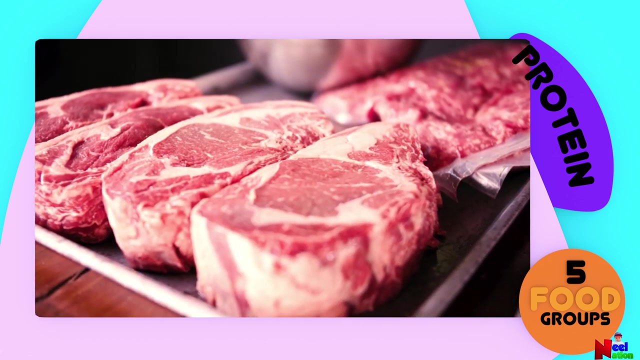 A whole grain contains all the three parts of the grain in its original proportions. A refined grain has the bran and germ removed, leaving just the endosperm. As a result, refined grains have less fiber and essential nutrients than the whole grain. Protein food includes all foods made from seafood, meat, poultry and eggs. 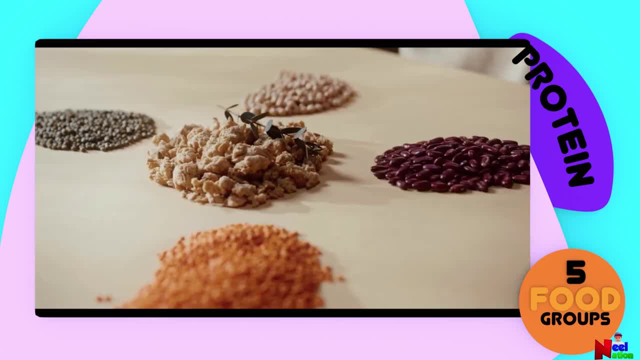 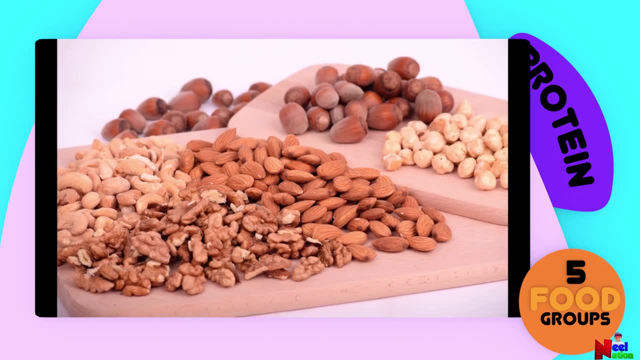 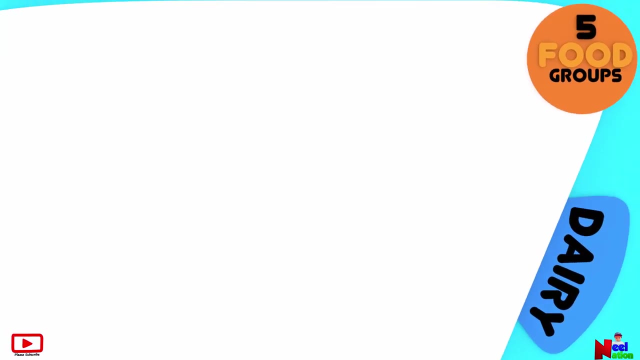 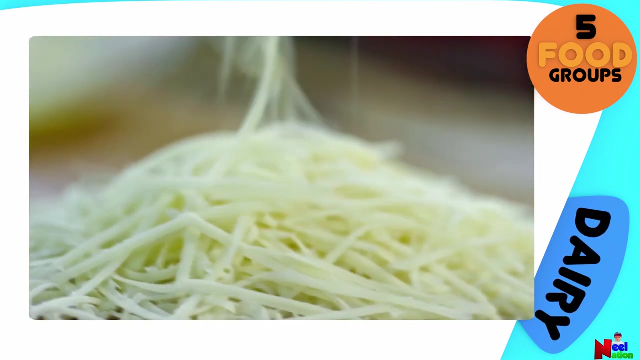 Beans, peas, lentils and nuts, seeds and soy products. A whole grain contains all the three parts of the grain. A whole grain contains all the three parts of the grain: Endosperm milk, yogurt cheese, lactose-free milk and fortified soya milk. The dairy group does 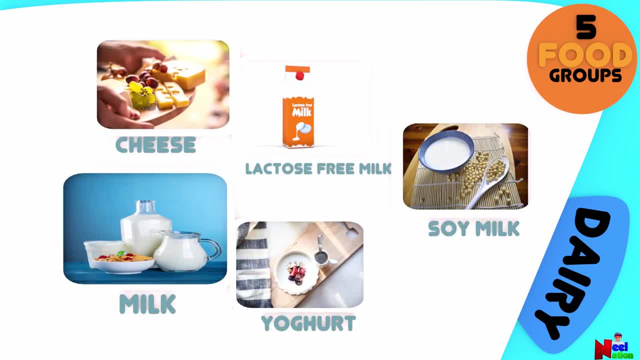 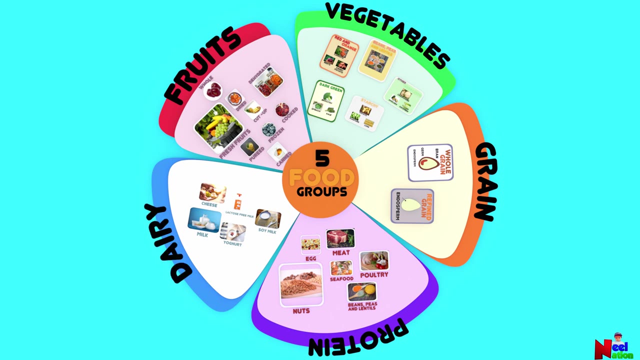 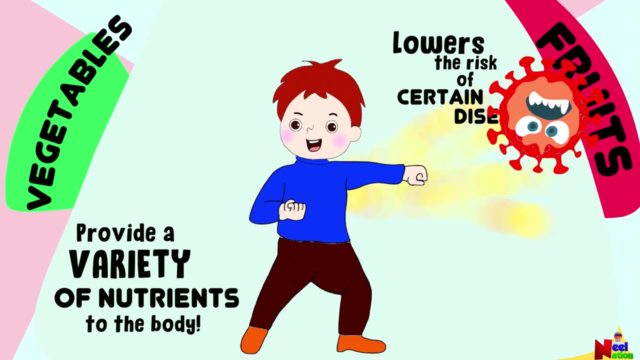 not include foods made from milk that have little calcium and a high fat content. Examples of these are cream cheese, sour cream, cream and butter. Fruits and vegetables provide a variety of nutrients to the body. People who eat fruits and vegetables as part of an overall diet may lower their risk for. 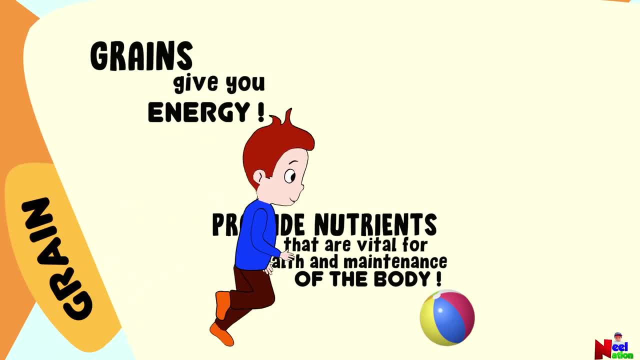 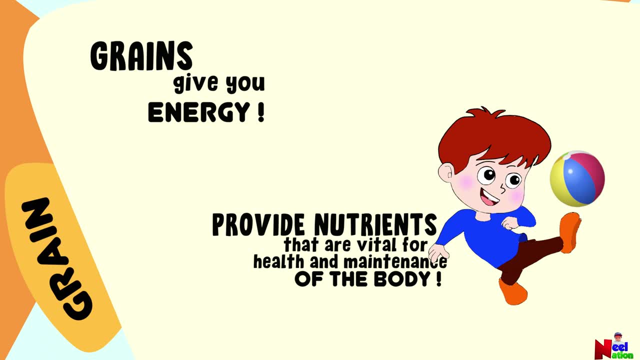 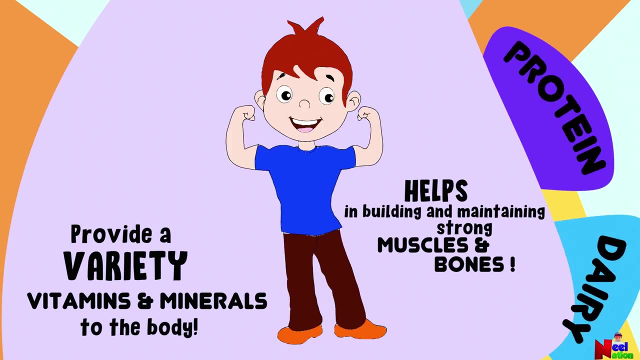 certain diseases. Grains give you energy and provide many nutrients that are vital for the health and maintenance of our body. Protein and dairy provide a variety of vitamins and minerals and help in building and maintaining strong muscles and bones. A healthy, balanced diet includes food from these five groups in the right quantities. So how much do you? 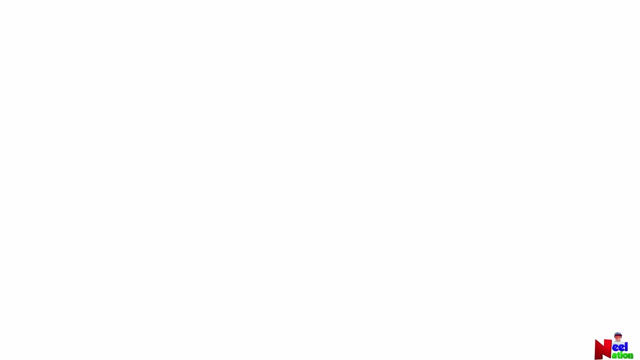 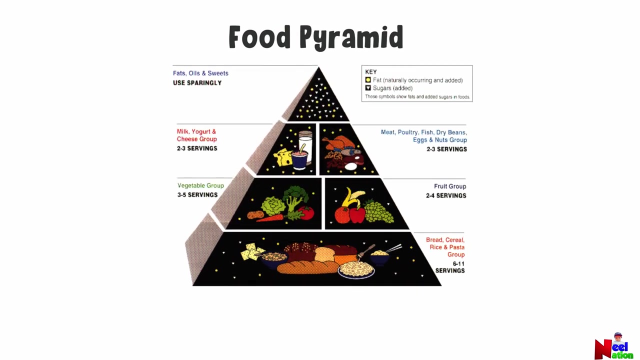 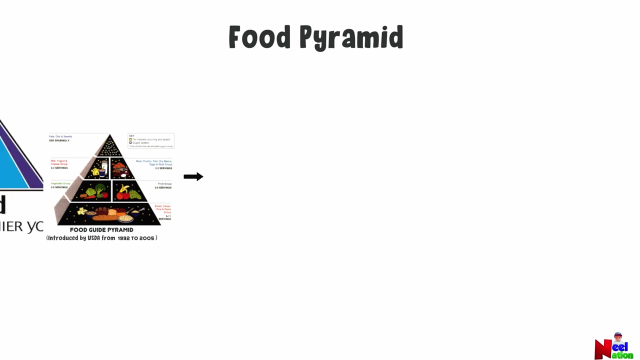 need from each food group To tell you the optimal number of servings to be eaten each day from each of the basic food groups, a food pyramid was introduced. This is a food guide pyramid introduced by United States Department of Agriculture in 1992.. It was later updated to MyPyramid in 2005..